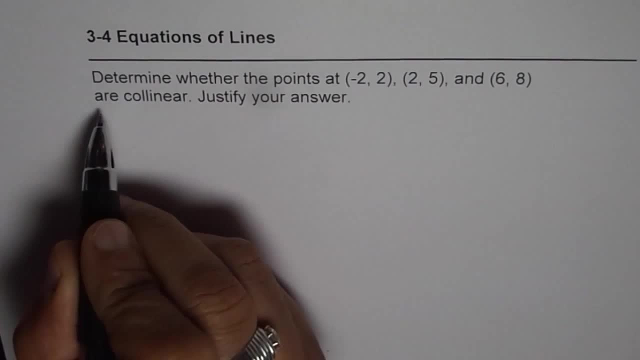 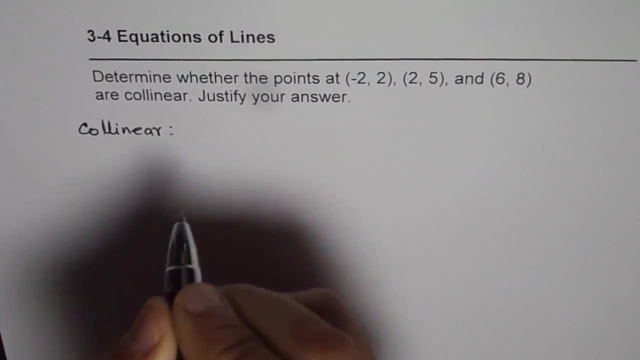 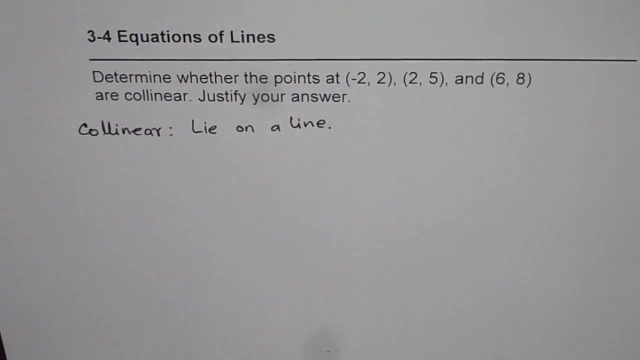 Justify your answer. So let us first understand what are collinear points. When we say collinear, that means the points which lie on a line. Those points are collinear. Now, to verify whether the given three points will lie on a line or not, what we should do is we should find: 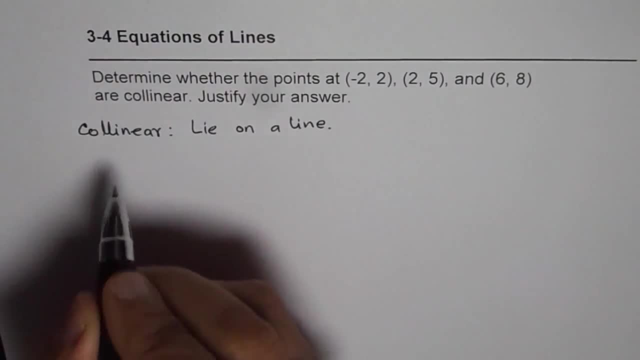 equation of line using any two points. So let us use two points which are minus 2, 2 and 2, 5, and find the points which lie on a line. So let us use two points which are minus 2, 2 and 2, 5. 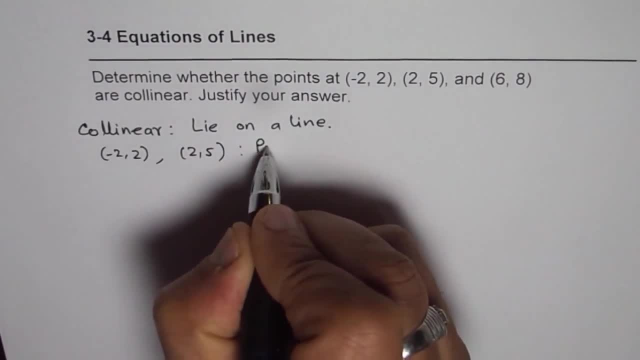 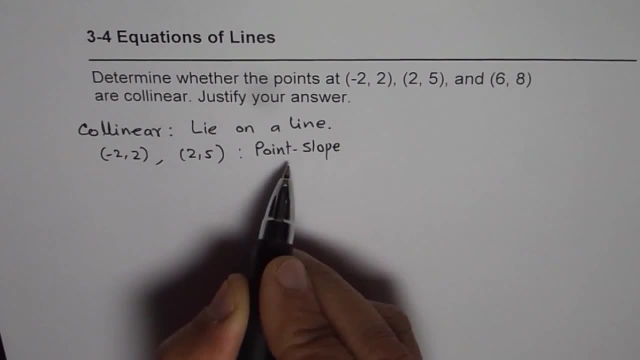 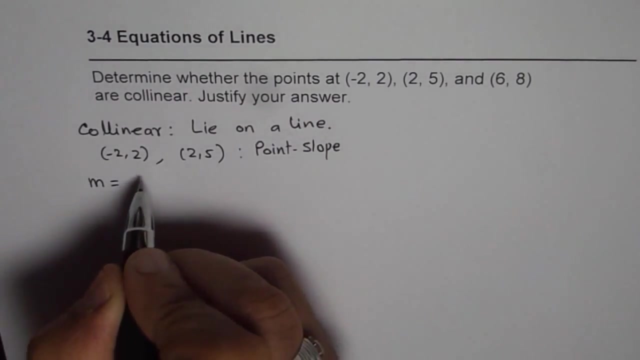 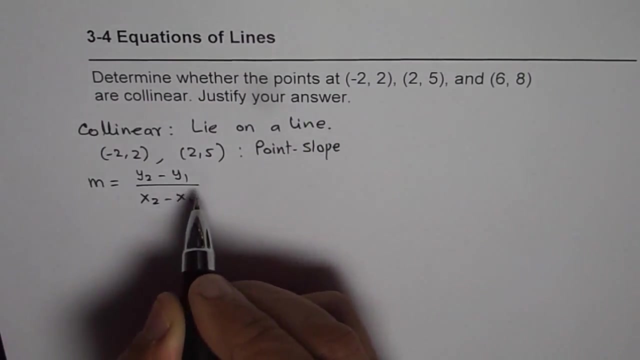 and find equation of the line and we will use point slope form of the equation. So in that equation, first we need to find the slope. We already know the points right. So the slope is using the slope formula, which is y2 minus y1 divided by x2 minus x1.. We can substitute these points: x1, y1, x2, y2. 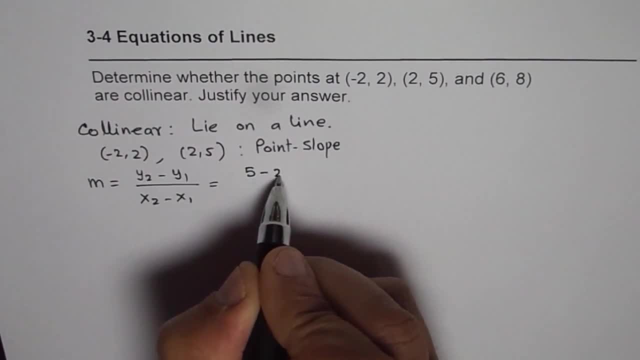 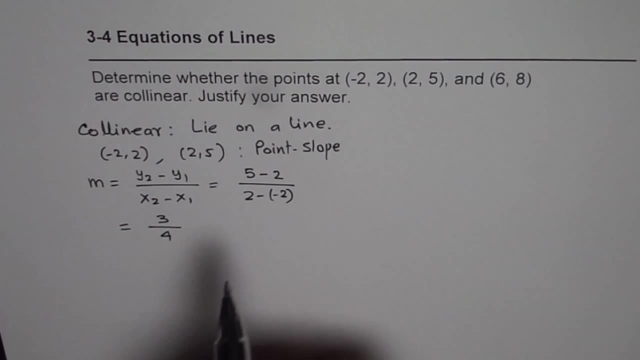 so y2 minus y1 will be 5 minus 2 divided by 2 minus minus 2, 2 minus minus 2.. So what we get here is 5 minus 2 is 3, and 2 minus minus 2 is 4.. So equation of the line now can be written in point. 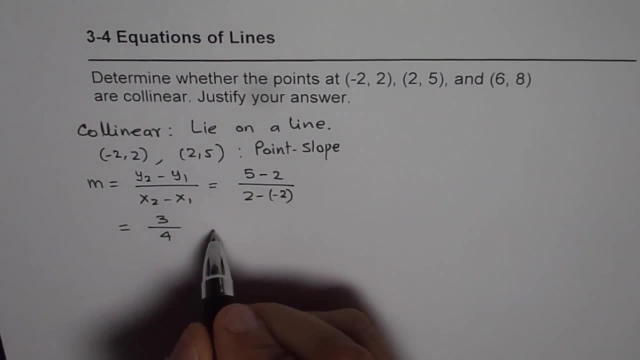 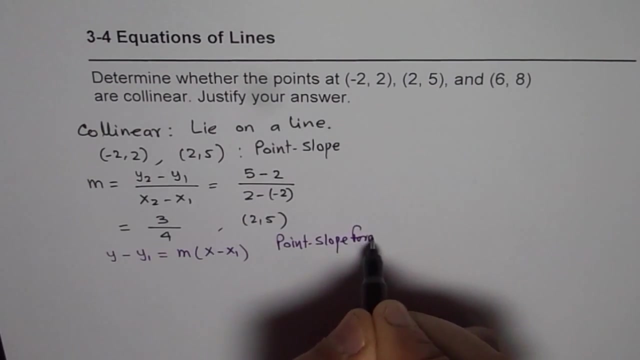 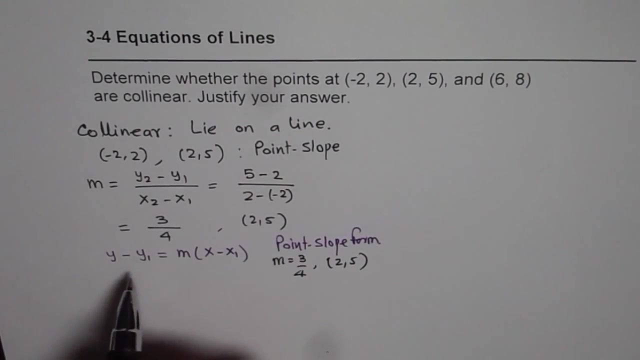 slope form, since we know the slope, And let us now consider the point which is 2, 5.. In point slope form the equation is: y minus y1 equals x minus y1. that is point slope form. Right now let us consider the point 2, 5.. So here we can consider slope n as 3 over 4 and the point as 2, 5.. So what? 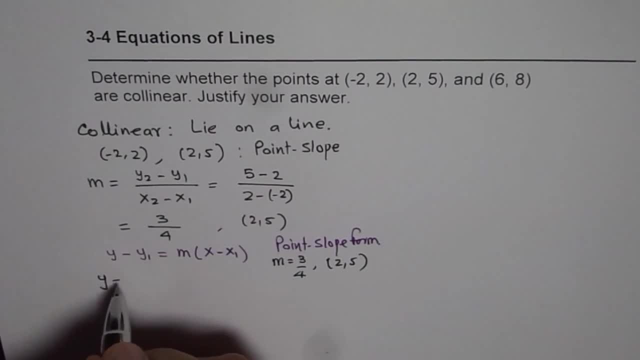 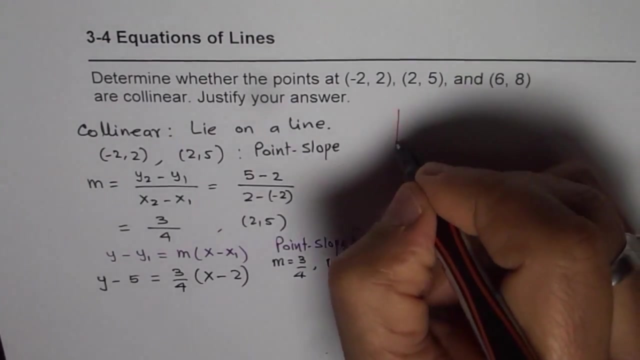 we get here is y values 5, so we get: y minus 5 equals to 3 over 4 times x minus 2.. So that becomes the equation of our line. Now we'll verify whether the third point, which is 6,. 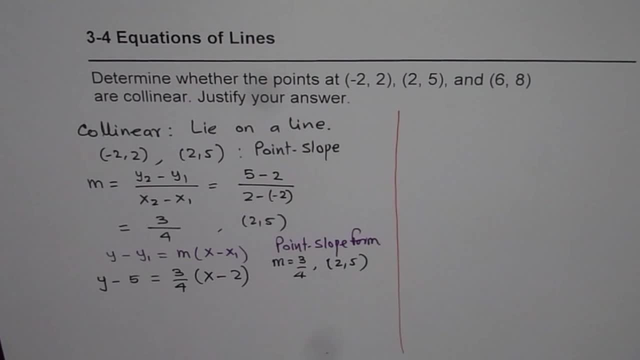 8, lies on this point or not. As you know from the definition of line, line will always contain a distinct. line will always contain two points, right at least? So those two points form one line. Now third point. let us check. So we have equation as y minus 5. 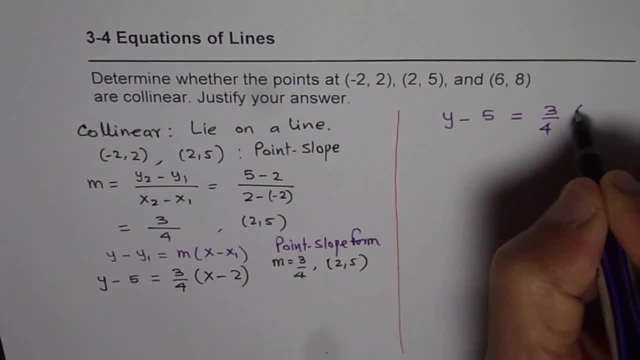 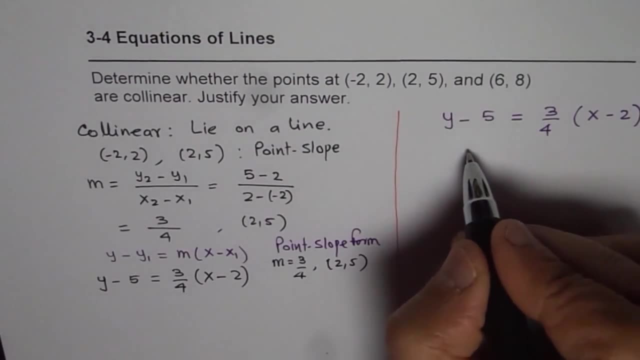 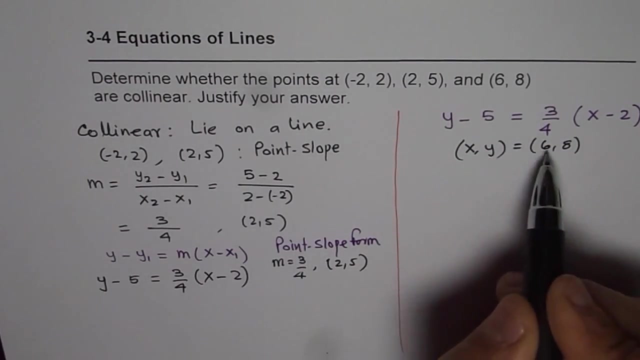 equals to 3 over 4, x minus 2.. And we need to verify that. the point 6, 8, so we have a point. let's call x, y is equals to 6, 8.. We need to verify whether it lies on this line or not. So let's solve for the left side. 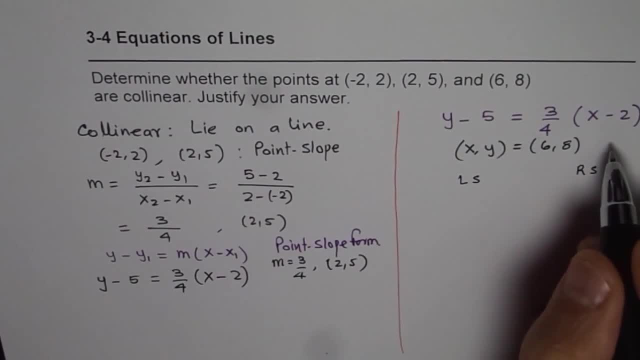 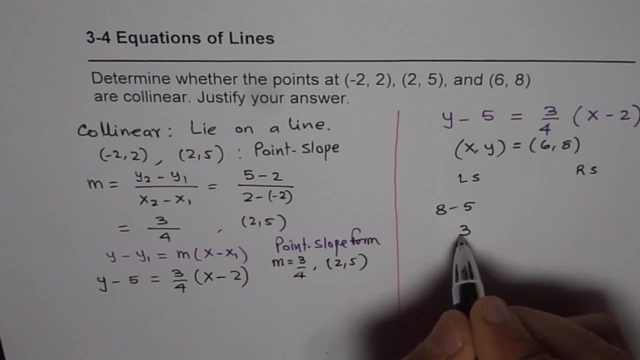 and the right side and check whether both are same or not. So y is 8, so 8 minus 5 is on the left side, which gives us 3.. On the right side we get 3 over 4, x value 6, 6. 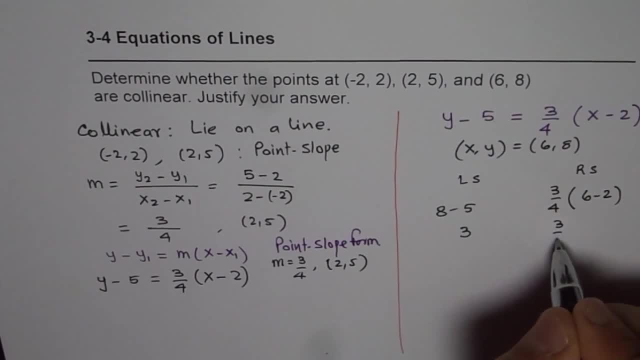 minus 2,, and that gives us 3 over 4,. 6 minus 2 is 4,, and this is also equals to 3.. Now we see that left side is indeed equal right, So therefore the point satisfies the equation. 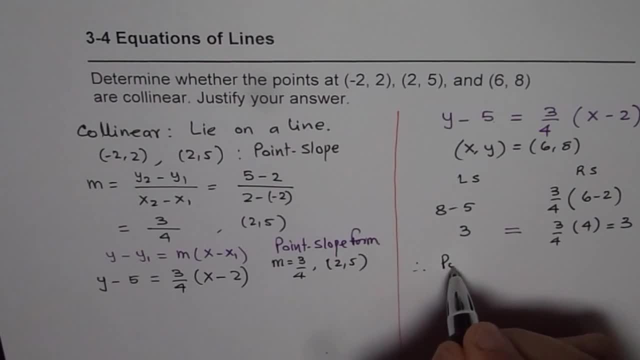 right, And therefore we can say that points are collinear. right, So the points are collinear, since all lie on the line Y minus 5 equals to 3 over 4, same line, right? That is how we can show that the three points 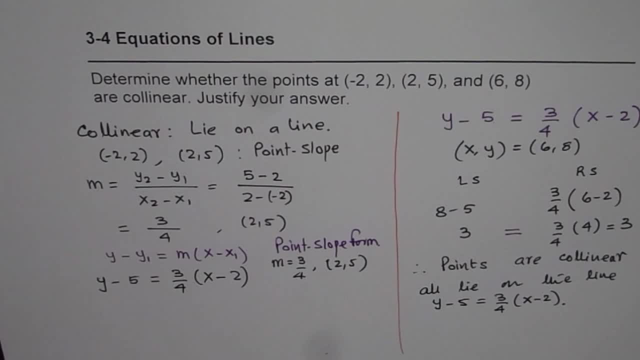 are collinear. I hope you understand the concept Well. the other way which you were telling was: you could find slope between two of these lines. right, finding slope between these two and these two. And if the slopes are same, then they are collinear. No, If the slopes 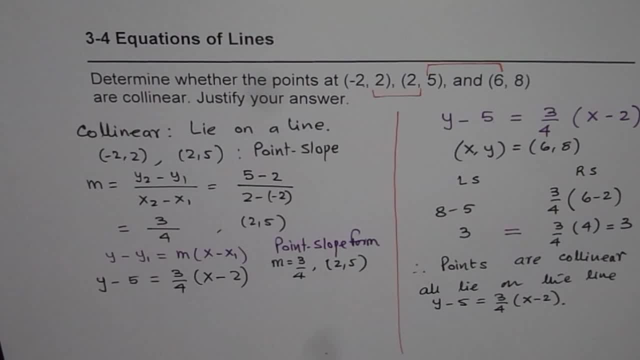 are same. they are only parallel. For collinear they have to lie on this line, right? So we have to lie on the same line, right? That is kind of important. So you have to write all these things and understand the whole concept to prove that any three points are. 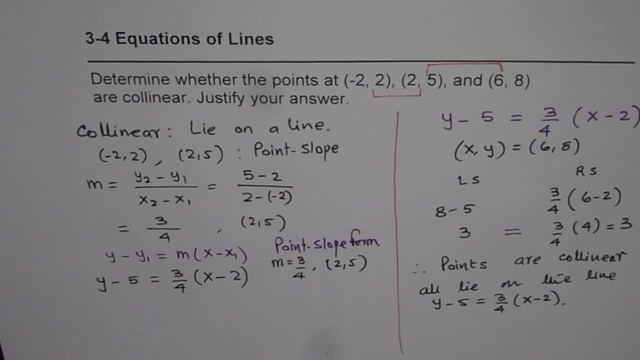 collinear. I hope it is clear to you. Thank you and all the best.